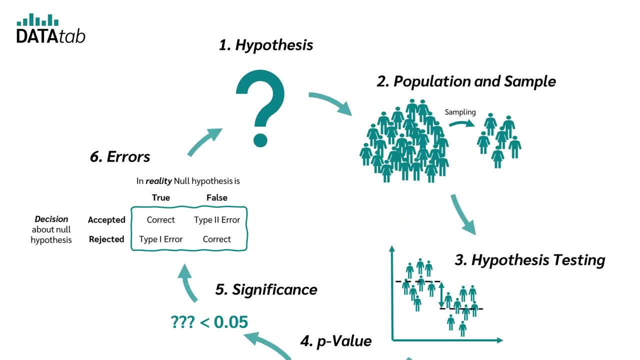 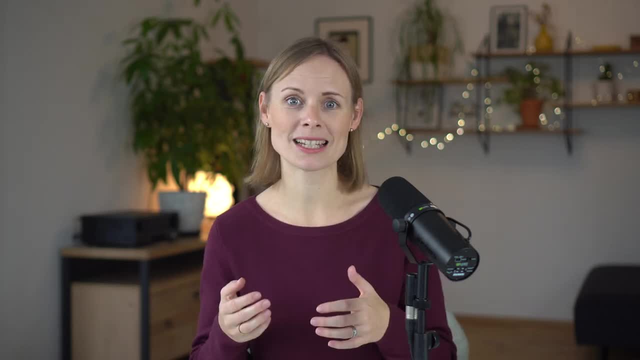 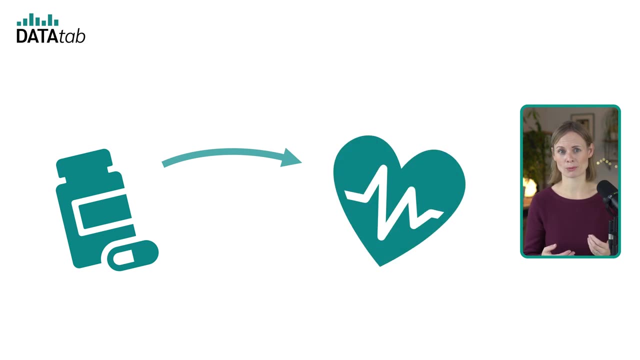 And here are the six steps: how to do that. Number one Hypothesis: First, of course, we need a statement, a hypothesis that we want to test. For example, we want to know whether a drug will have a positive effect on blood pressure in people with high blood pressure. But what's next? In our 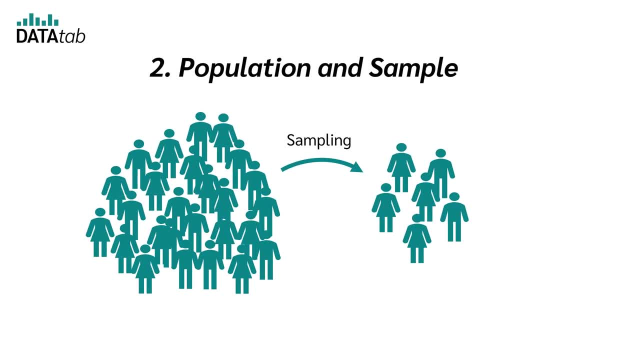 hypothesis. we have stated that we would like to study people with high blood pressure, So our population will have a positive effect on blood pressure in people with high blood pressure. The population is all people with high blood pressure in, for example, the US. Now we want to. 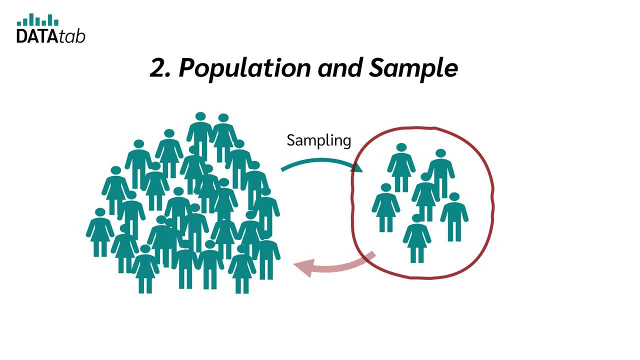 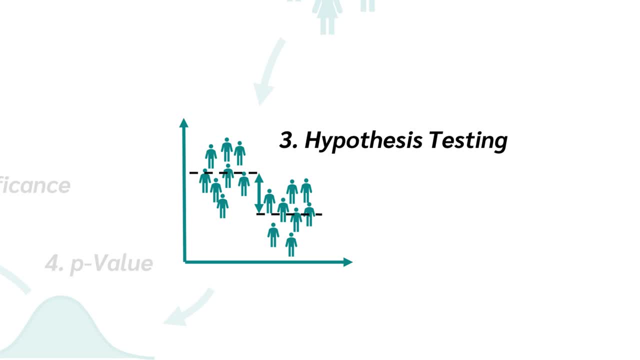 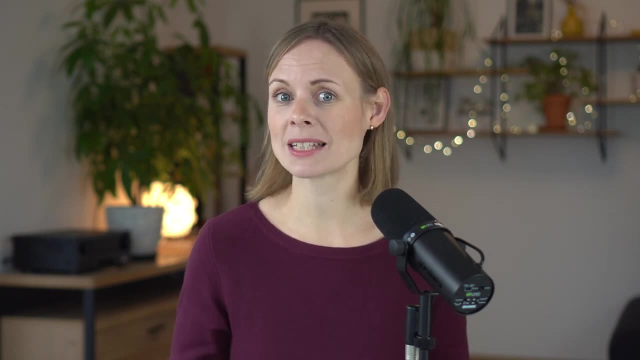 use this sample from that population to make a statement about the whole population. But how do we do that? For this we need a hypothesis test. Hypothesis testing is a method for testing a claim about a parameter in a population using data measured in a sample. Great, that's exactly. 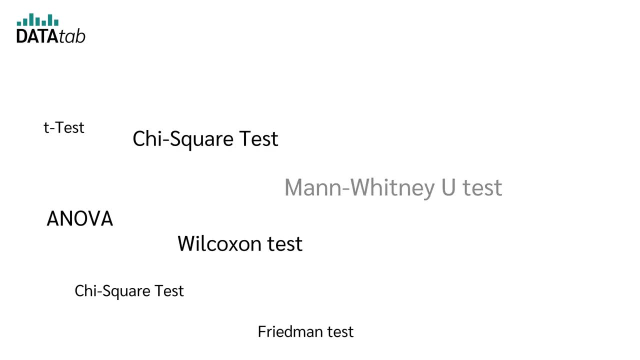 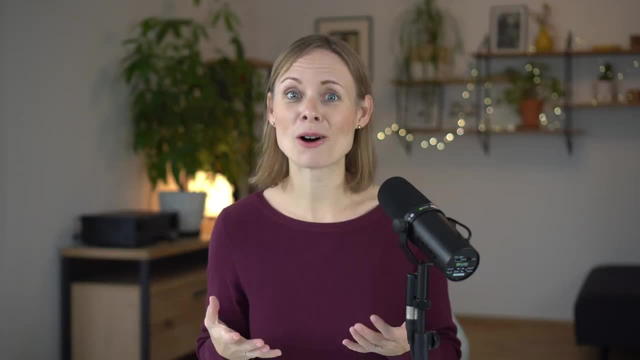 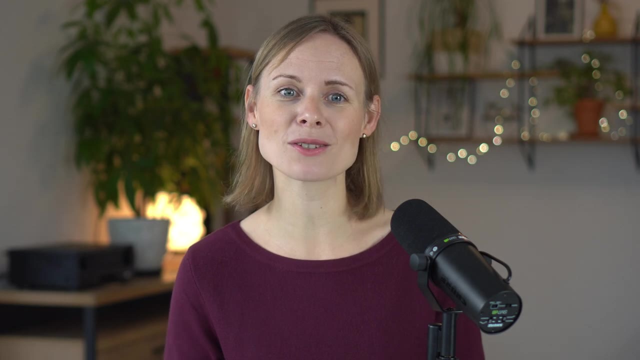 what we need. There are many different hypothesis tests. At the end of this video, I will give you a guide to help you find the right test. But how does a hypothesis test work? When we conduct a hypothesis test, we start with a research hypothesis, also called alternative hypothesis. This is the 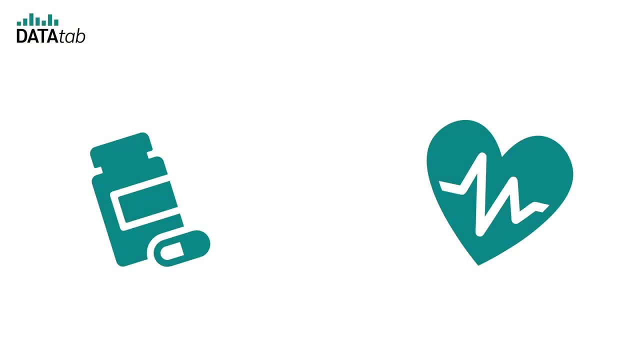 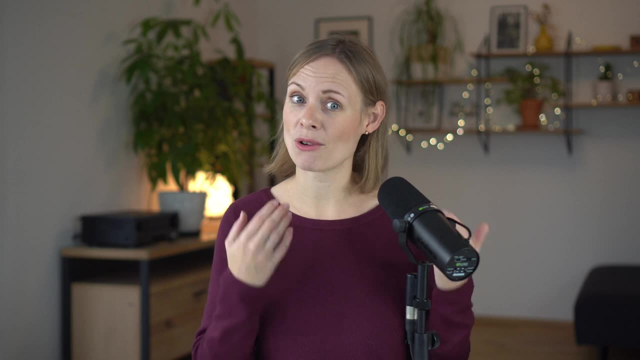 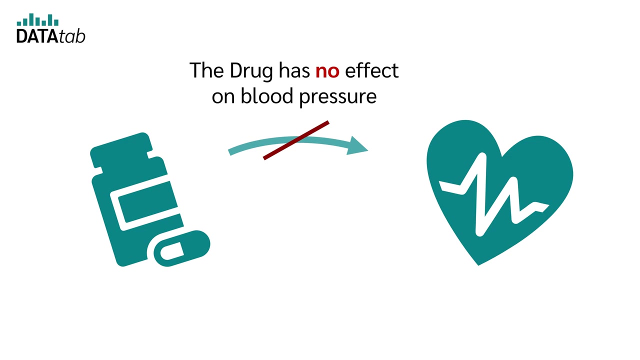 hypothesis we are trying to find evidence for. In our case that drug has an effect on blood pressure. But we cannot test this hypothesis directly with a classical hypothesis test, So we test the opposite hypothesis, that the drug has no effect. So we first assume that the drug has no effect in the 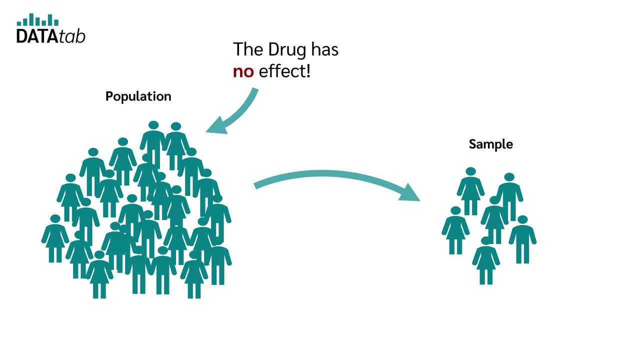 population. If we now take a random sample and it turns out that the drug has a large effect in this sample, then we can ask how likely it is to draw such a sample or one that deviates even more, if the drug actually has no effect. If this probability is very low, we can ask ourselves. 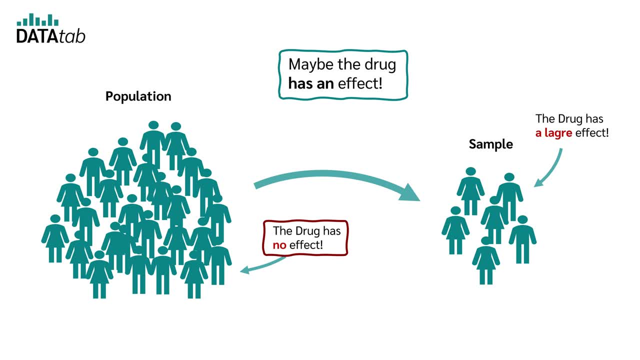 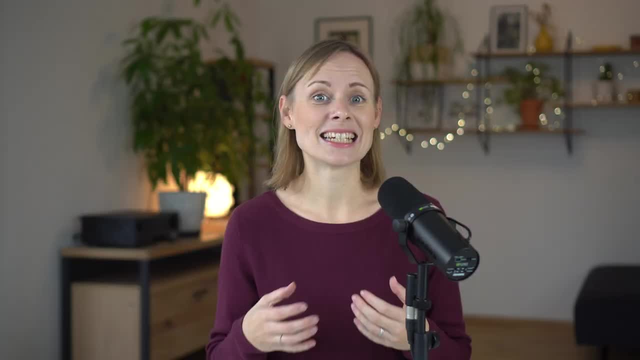 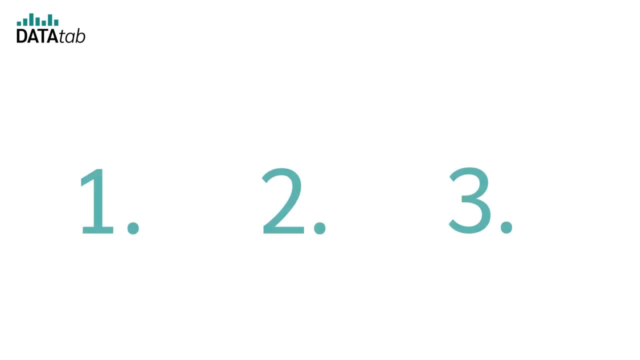 maybe the drug has an effect in the population And we may have enough evidence to reject the null hypothesis that the drug has no effect, And it is this probability that is called the p-value. Let's summarize this in three simple steps. Number one: the null hypothesis states that 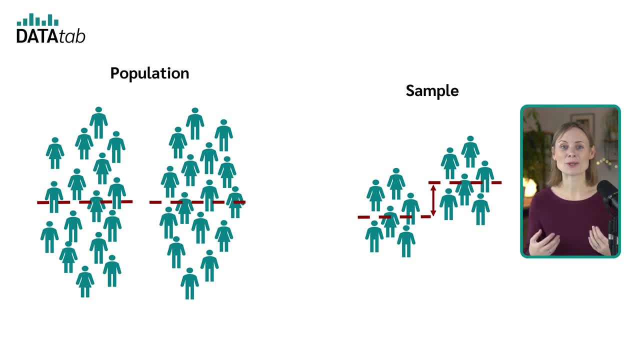 there is no difference in the population. Number two: the hypothesis test calculates how much the sample deviates from the null hypothesis. Number three: the p-value indicates the probability of getting a sample that deviates as much or more than our sample, under the assumption that the 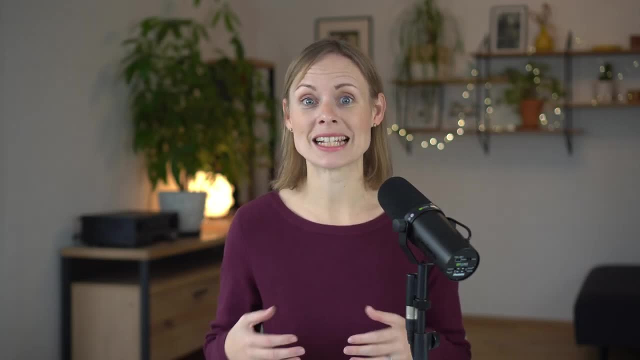 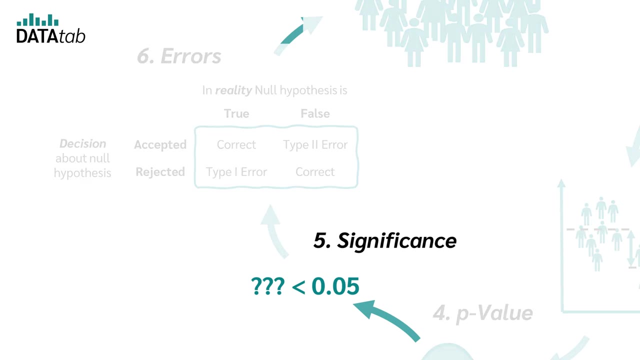 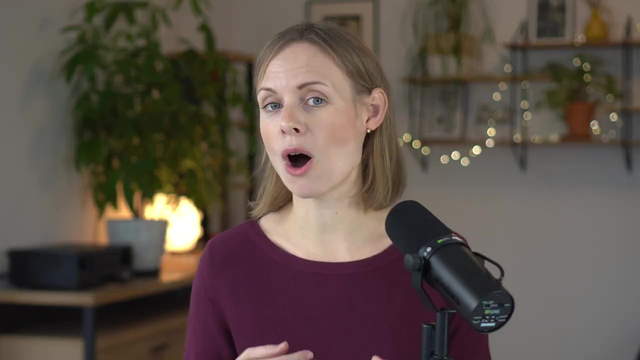 null hypothesis is true, But at what point is the p-value small enough for us to reject the null hypothesis? This brings us to the next point: statistical significance. If the p-value is less than a predetermined threshold- often 0.05, the result is considered statistically significant. 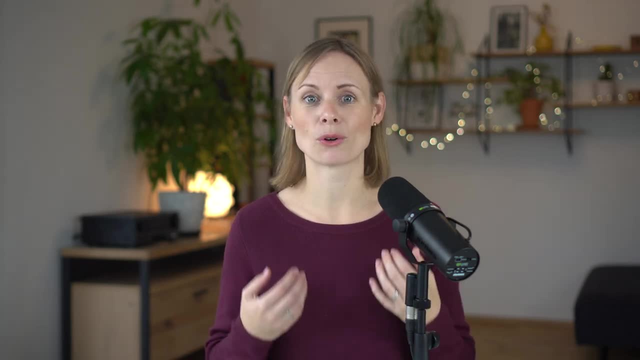 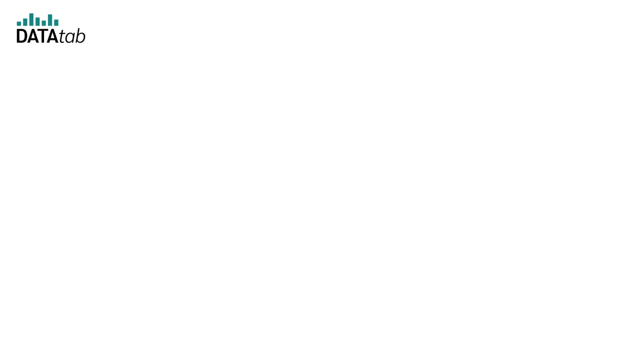 meaning that the result is unlikely to have occurred by chance alone and that we have enough evidence to reject the null hypothesis. Therefore, a small p-value suggests that the observed data or sample is inconsistent with the null hypothesis, leading us to reject the null. 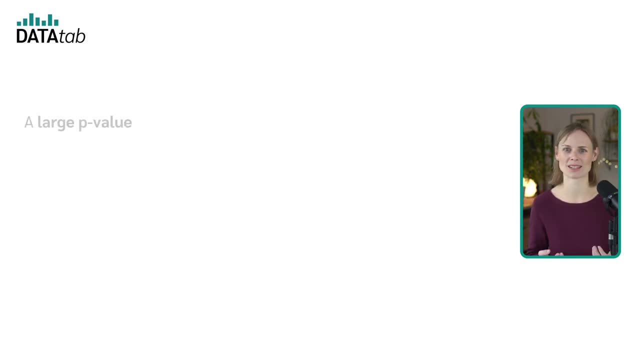 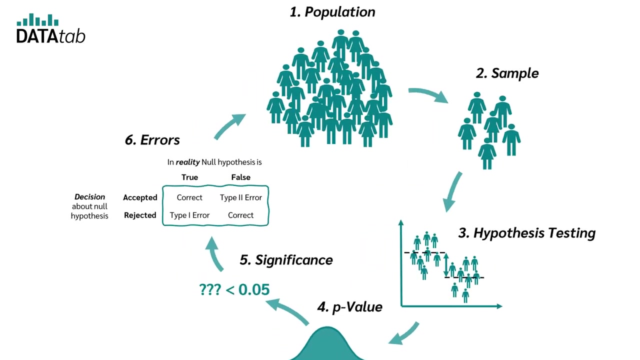 hypothesis in favor of the alternative hypothesis. A large p-value suggests that the observed data is consistent with the null hypothesis and we will not reject it. Before I show you how to find a suitable hypothesis test, here is the important last point. There is always a risk of making an error. 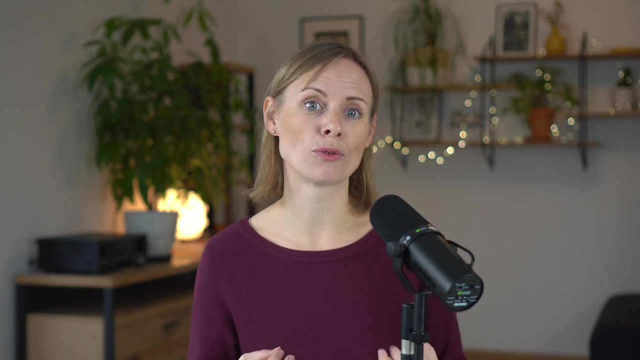 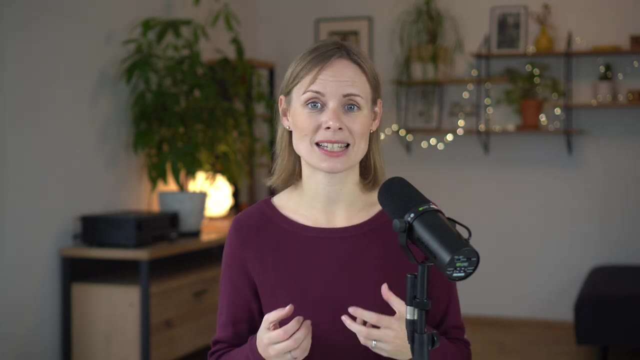 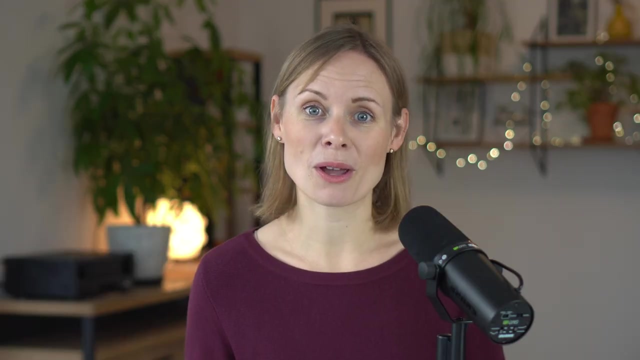 A small p-value does not prove that the alternative hypothesis is true. It is only saying that it is unlikely to get such a result or a more extreme when the null hypothesis is true, And the other way around. a large p-value does not prove that. 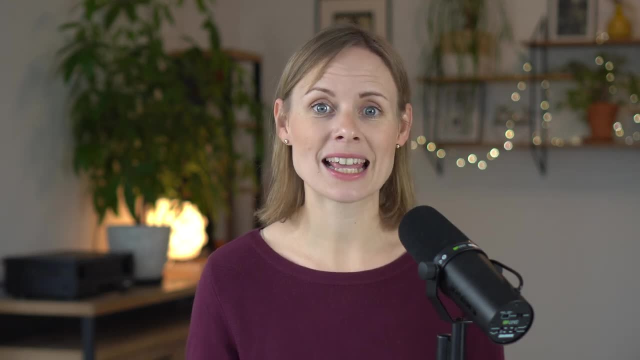 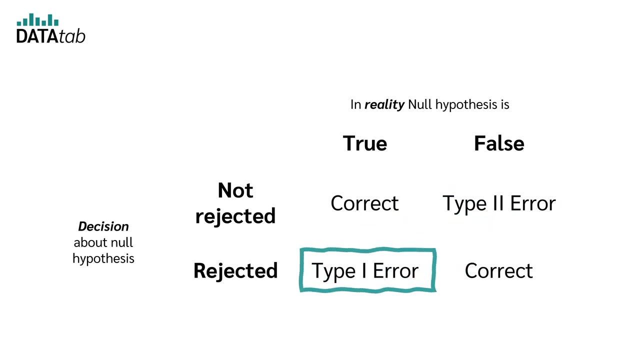 the null hypothesis is true, It is only saying that it is likely to get such a result or a more extreme when a null hypothesis is true. So there are two types of errors, which are called type I and type II error. Let's start with the type I error. 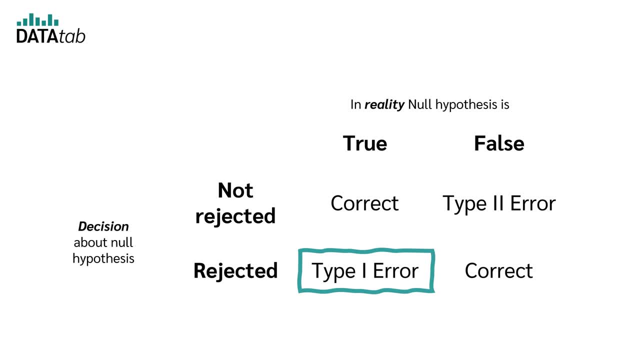 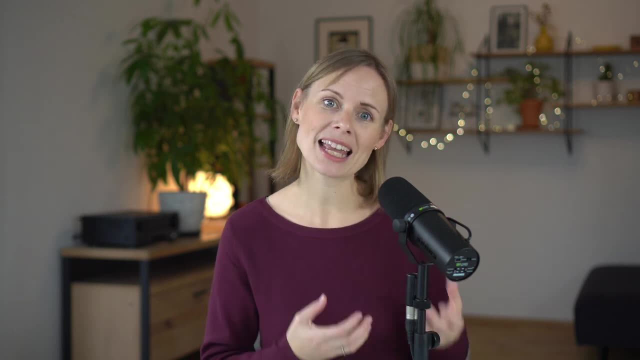 In hypothesis testing, a type I error occurs when a true null hypothesis is rejected. So in reality, the null hypothesis is true, but we make the decision to reject the null hypothesis. In our example, this means that the drug actually did not reject. 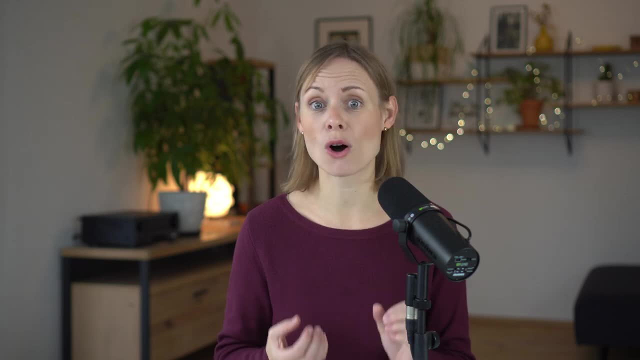 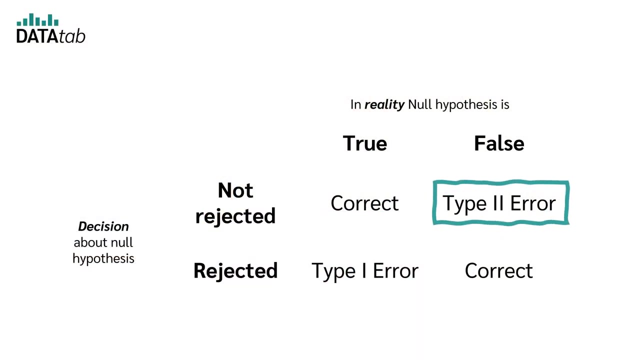 work, but our sample happened to be so far off the true value that we mistakenly thought the drug was working. And a type II error occurs when a false hypothesis is not rejected. So in reality, the null hypothesis is false, but we make the decision to not reject the. 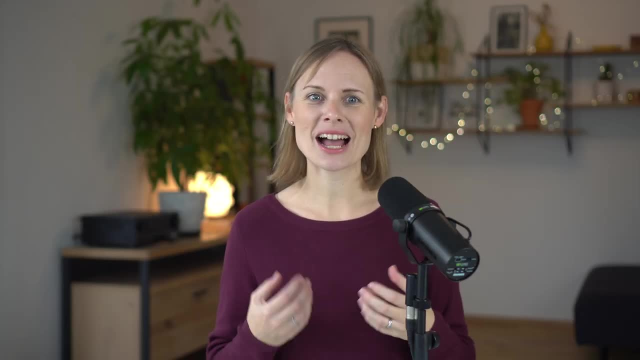 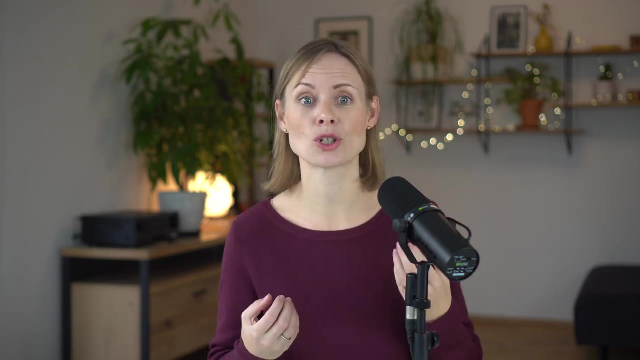 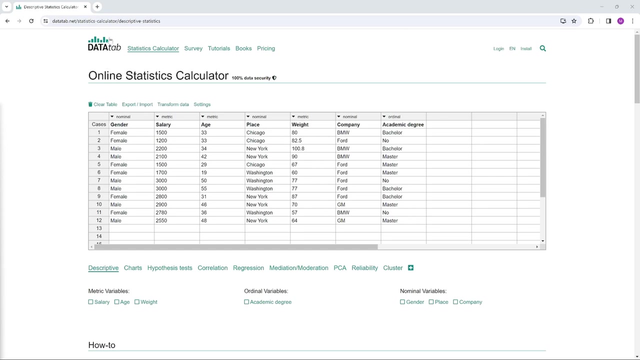 null hypothesis. In our example, this means the drug actually did work, but it was just a coincidence that the sample taken did not show much difference and we mistakenly thought the drug was not working. And now I'll show you how Datadep helps you find a suitable hypothesis test and of 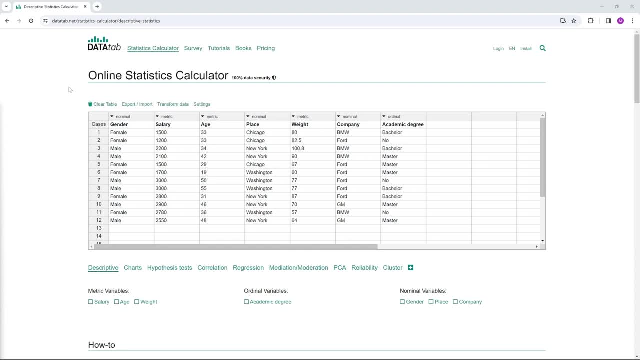 course, calculates it and interprets the results for you. Let's go to datadepnet and copy your own data into this table. Now the variables appear down here. Datadep automatically tries to determine the correct scale. You can also change it up here. 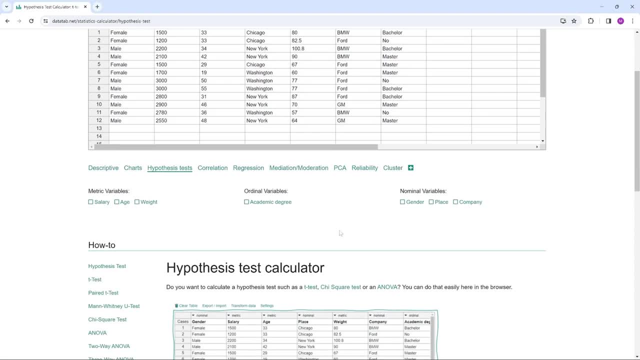 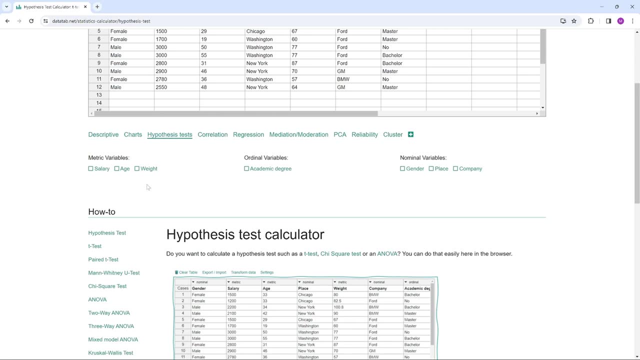 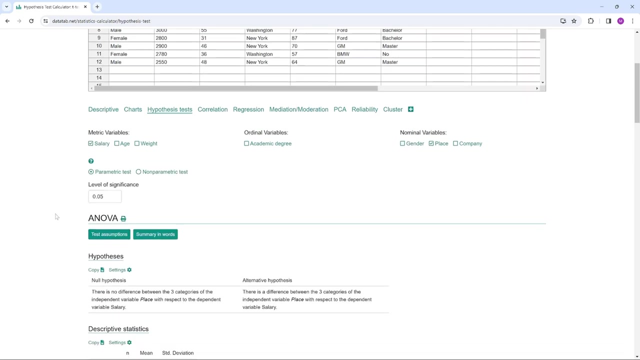 Now just click on Hypothesis testing and select the variables on which we want to calculate a hypothesis test. Datadep will then suggest a test, For example, in this case, a chi-square test or, in that case, an analysis of variance. 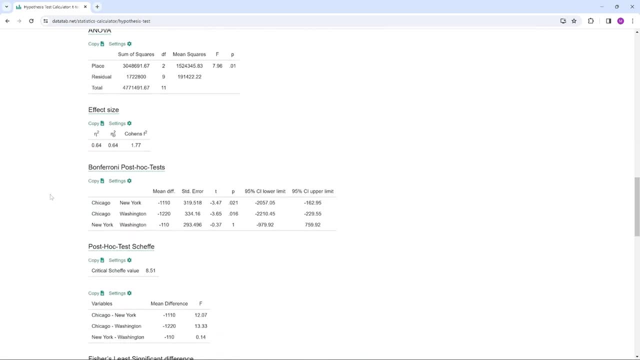 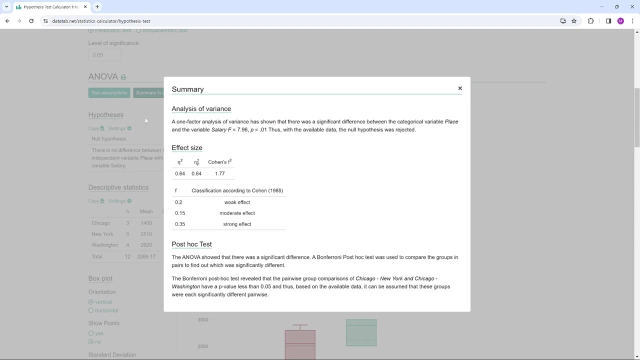 Then we will see the hypotheses and then the results. If you're not sure how to interpret the results, click here. And now we have a hypothesis test. Let's see how it works. Click on Summary- Inverts Further you can check the assumptions and decide whether you want to calculate a parametric. 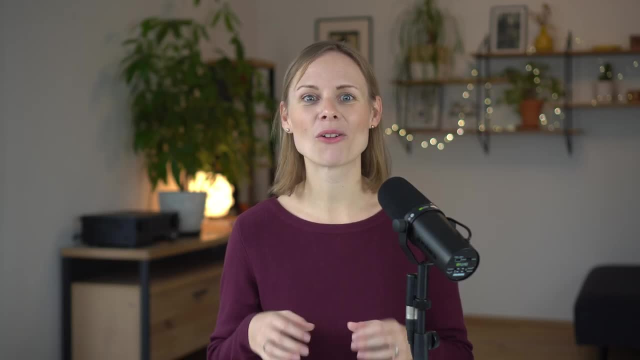 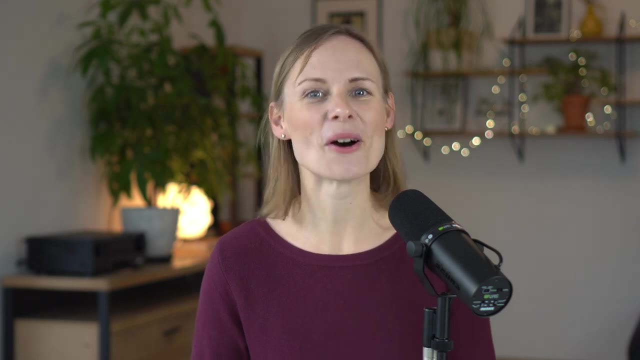 or a non-parametric test. You can find out the difference between parametric and non-parametric tests in my next video. Thanks for watching and I hope you enjoyed the video.